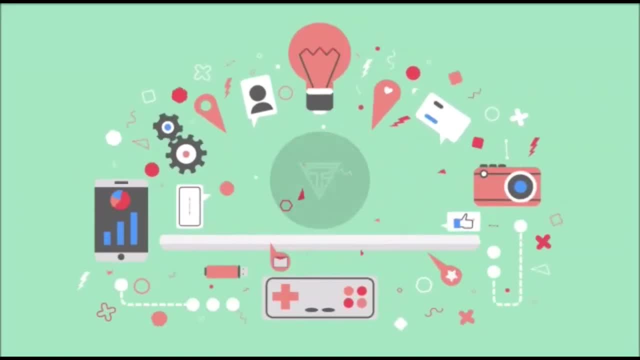 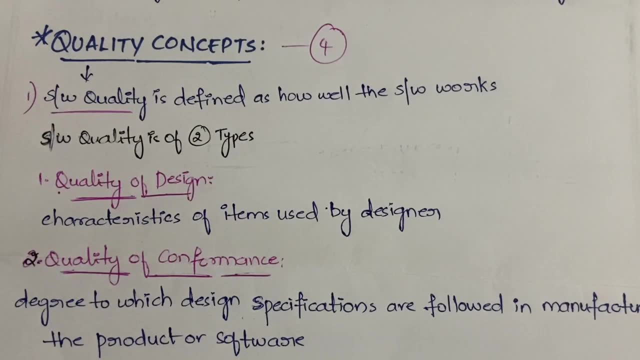 Hello everyone, welcome back to my YouTube channel, Trouble Free. In today's video I'm going to explain you about the quality concepts in the subject of software engineering. So we have four quality concepts. We are going to discuss about each of them in detail in this video. And before going into the video, let me tell you something. I have started a new channel, new study abroad content channel. I'll give you the link of the. 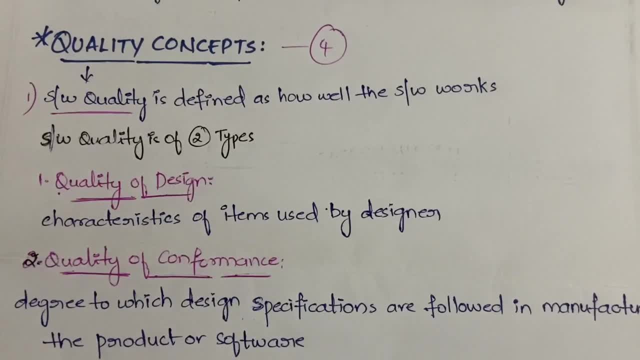 channel in the description. You can check it out if you're interested. So let's get into the video now. So actually we have four software concepts, Got it? Sorry? quality concepts. The first one is quality, Second is quality control, Third is quality assurance And the fourth is a quality, cost of quality. Okay, quality, quality control, quality assurance and cost of quality. These are the four things we have. Okay, in that the first one is a software quality. How do you define software quality as How? 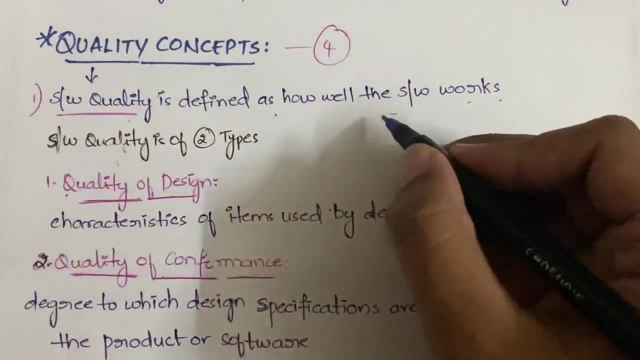 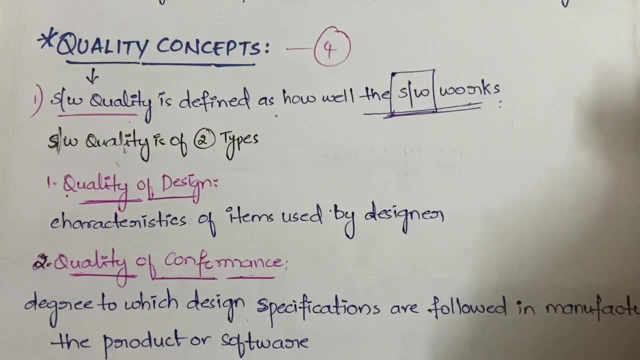 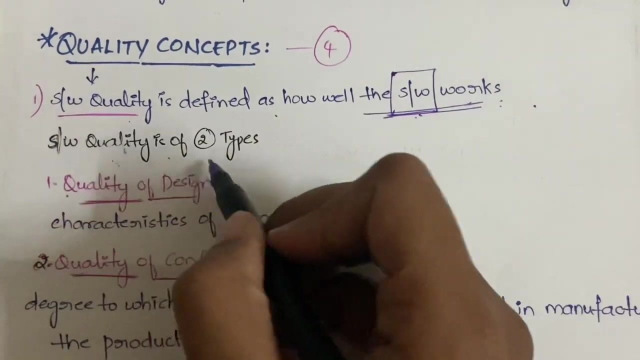 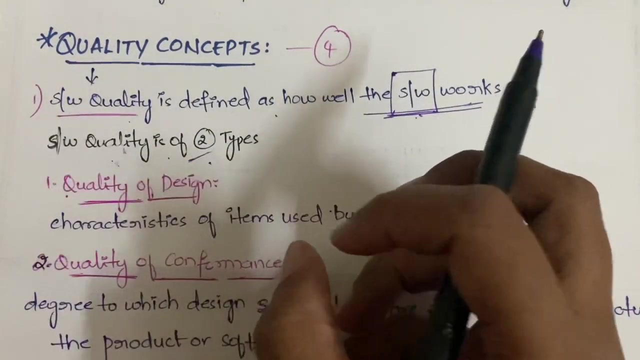 well the software works. The software quality is defined as how well the software works. that is, whatever software we have prepared or we have generated, produced, whether that software is working well or not. Okay, that's all. Next, again in software quality, we have two types In general. also, quality is what that only right. So for whatever purpose we bought an item, whether that item is serving us that purpose or not Right Now in software quality, you 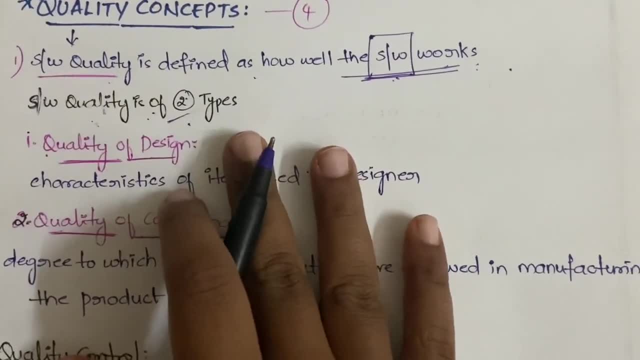 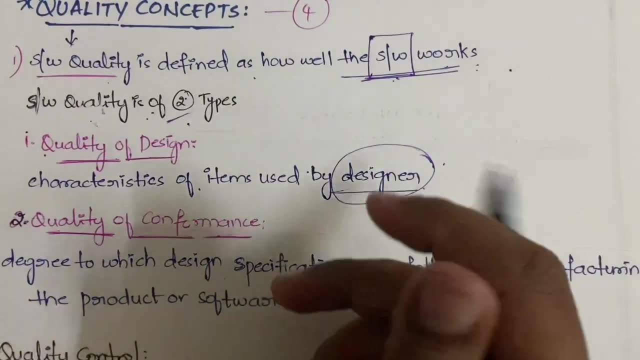 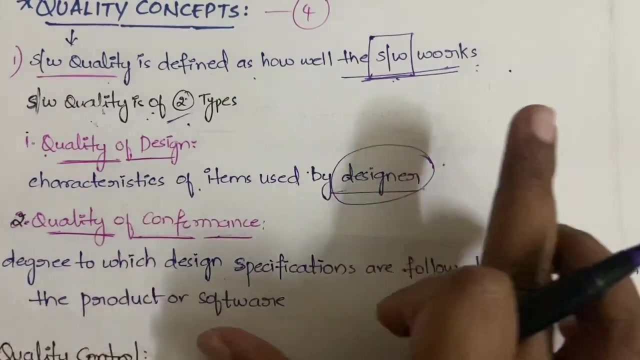 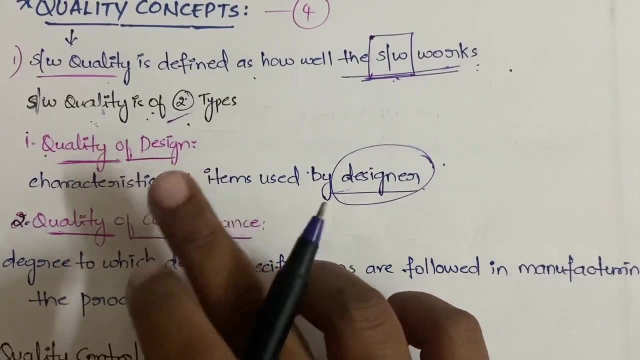 have two types of quality. Okay, first one is quality of design, which means characteristics of item used by the designer. So whoever is designing the software, that person, which quality of items he is using, the characteristics of the items used by the designer, whether he is using good quality tools or bad quality tools, highly secured one, you know, highly flexible one, all all those things will be seen here, the items or you can simply to understand, you can use the word 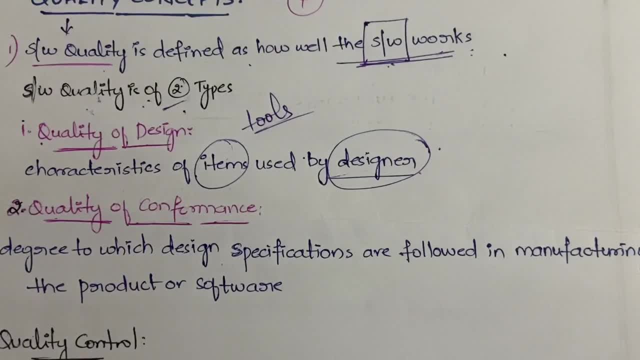 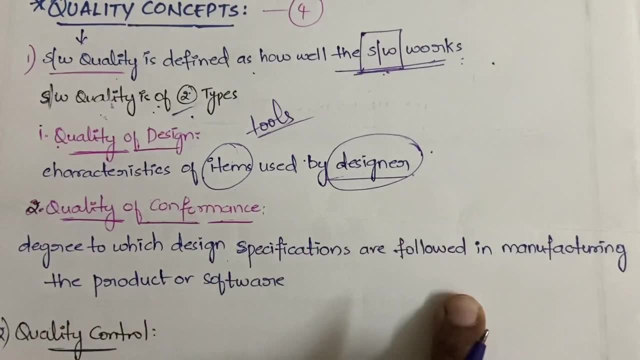 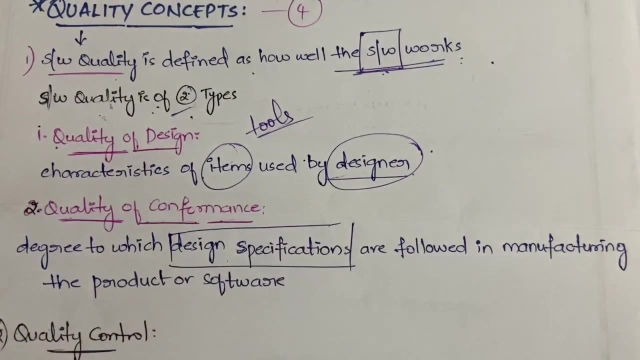 tools also here. Okay, next is quality of conformance. Quality of conformance is nothing but degree to which design specifications are followed in manufacturing the product or a software. So you will have certain design specifications, right, Like the design has to be in such a way: a design has to be a triangular one or a circle one or a square one, and the design has to be very simple, or it has to be complicated so that nobody can understand. So the degree 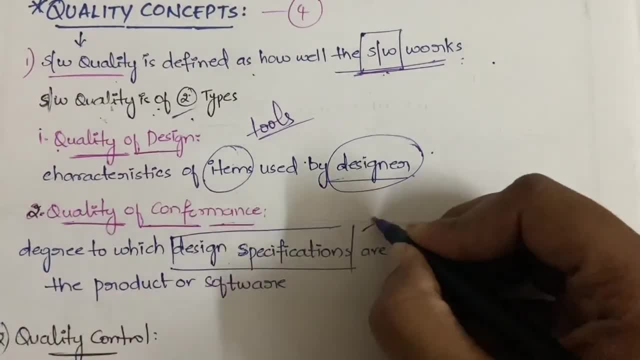 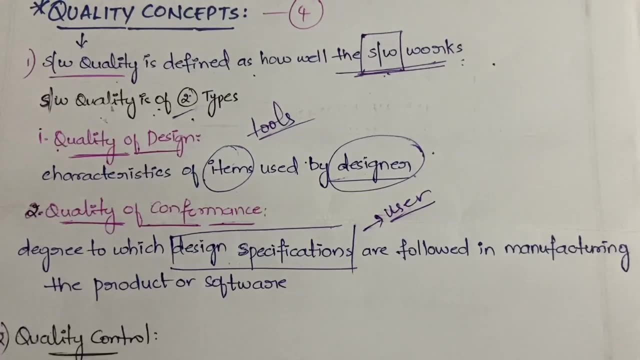 to which the design specifications which are defined by the user- okay, which are defined by the user- are followed in manufacturing the software or a product got it. that is what quality of conformance. whether you are following everything which is set by user or not, that is what quality of conformance. quality of design is nothing but what tools you are using to design. 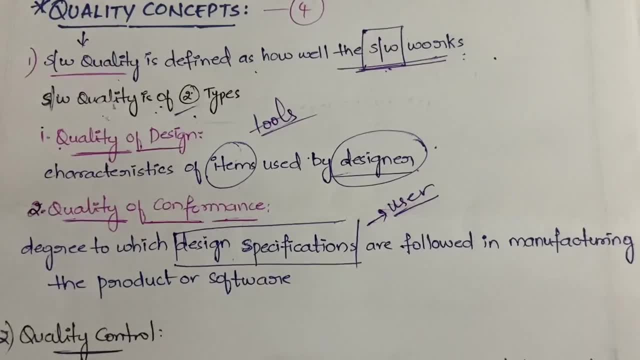 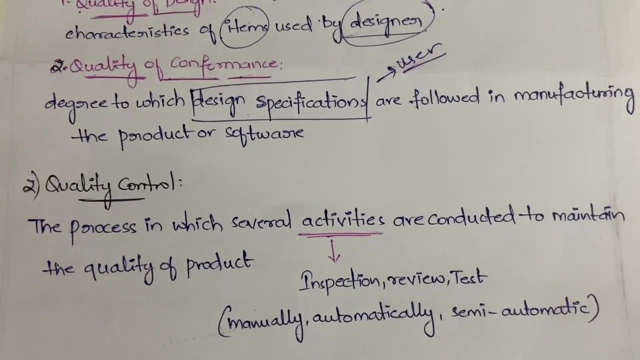 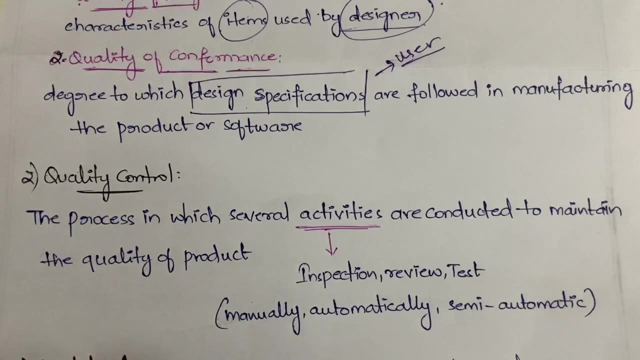 the quality of those tools right next. so done now. second, quality control. the first is quality- software quality, and that is done- and the next is quality control. it is very easy. so quality control is nothing, but it is a process in which several activities are conducted to maintain the 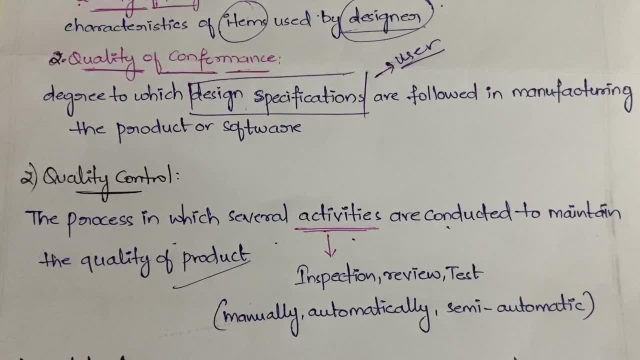 quality of the product. that is, you are controlling the quantity quality, how you are controlling the quality, you are performing several activities and those several activities are nothing, but it could be inspections, it could be reviews or it could be tests, anything. okay, inspections in the sense when the product is being manufactured during the 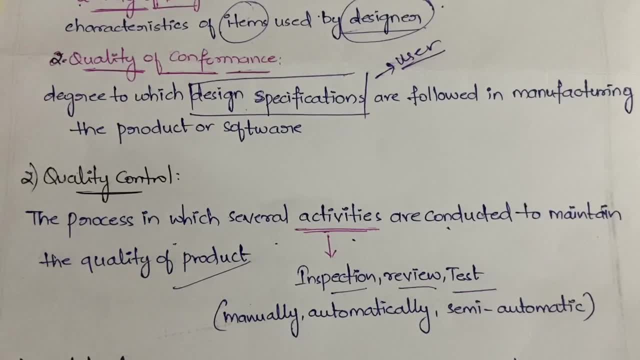 manufacturing itself, during the production itself. you will be going and you will be testing the software. you will be inspecting review in the sense, once it is done and once it is submitted to the reviewer, then you will be doing the review activity right, and test is nothing but once. 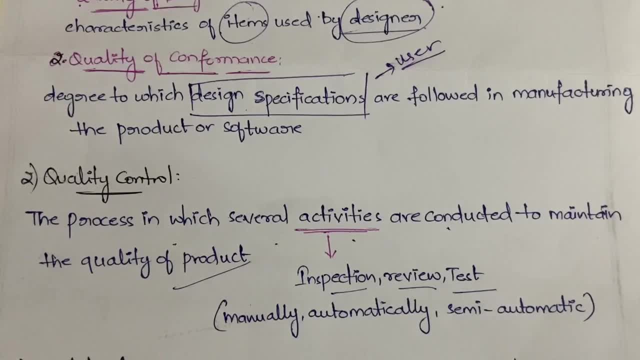 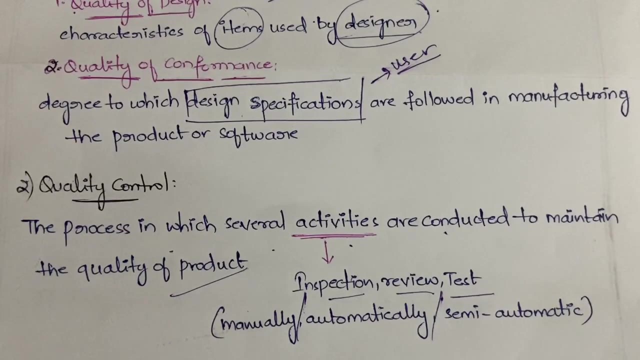 everything is finished, the software will move to the testing phase. right now, these activities- the inspection, review and test. they can be either done manually or automatically or semi-automatically, that is, using both manual and automatic techniques. got it. so this is quality control. quality control is nothing, but it is the process in which we do some activities in order to maintain the quality. 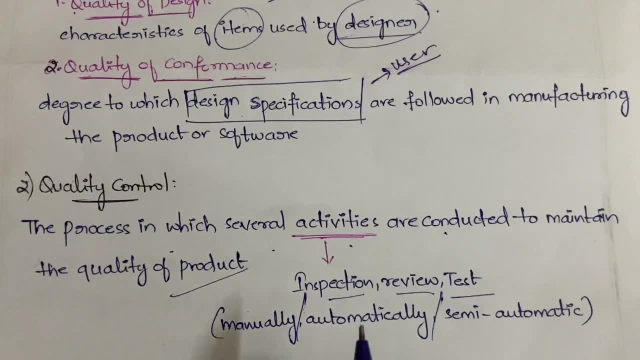 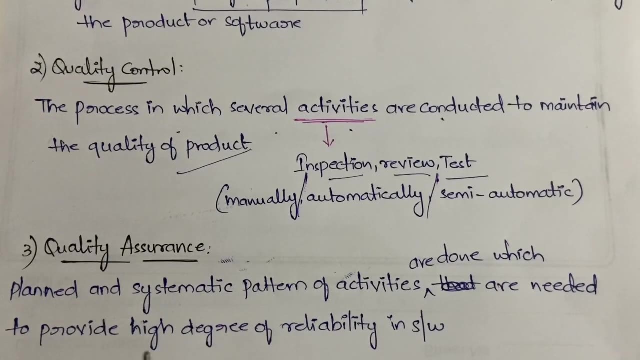 of the software got it and those activities could be inspection or review or test and they can be done as automatic or semi-automatic or manual done now. after this we have the quality assurance. so in quality assurance- it is also the third software quality concept, it is a planned and systematic pattern of activities are done. so here we planned and 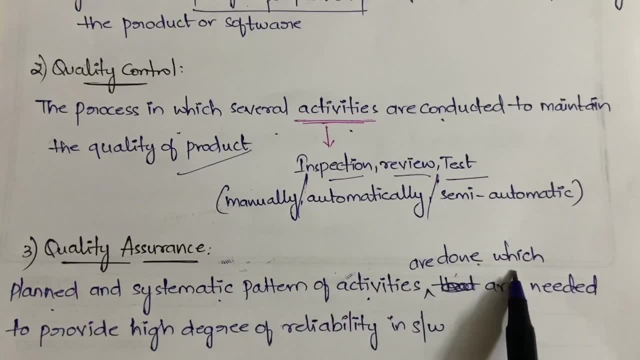 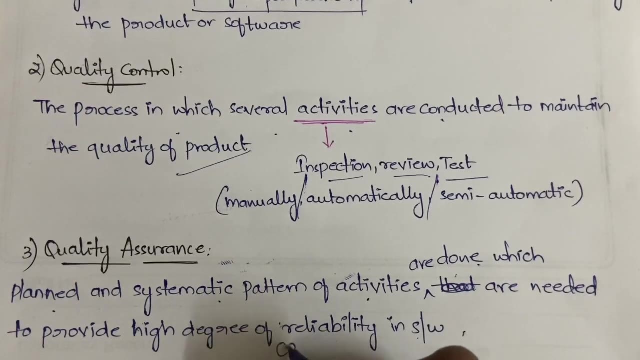 systematic pattern of activities are done. why? because they are needed to provide high degree of reliability in the software. okay, we do some activities which are required to provide high degree of reliability in the software. that is, high degree of reliability is nothing but the confidence on the software you can say confidence. okay, so we. 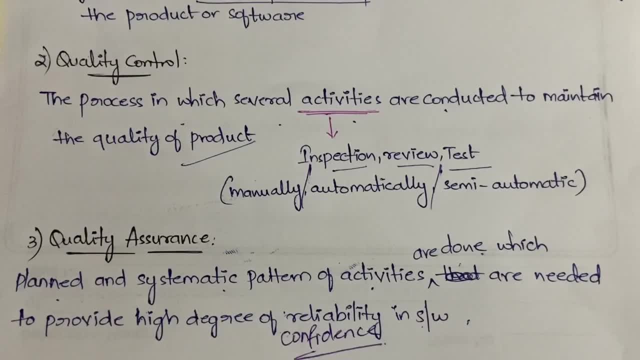 can depend on this software. okay, so this software is secured, this software is complete, like that. in order to completely get a confidence or get reliability on that software, we perform quality assurance, assurance in the sense the word itself says: right. so here we do some planned and systematic. 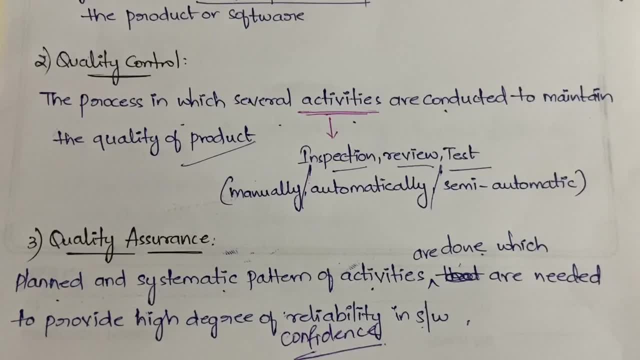 pattern of activities got it. so this is about the quality assurance. so, as i said, we have four quality concepts: software quality is done, quality control is done and quality assurance is done. quality assurance is, that's all same simple. okay. now we have the fourth one, which is nothing but the cost. 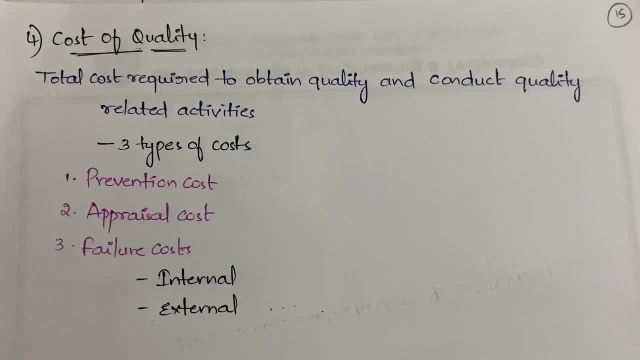 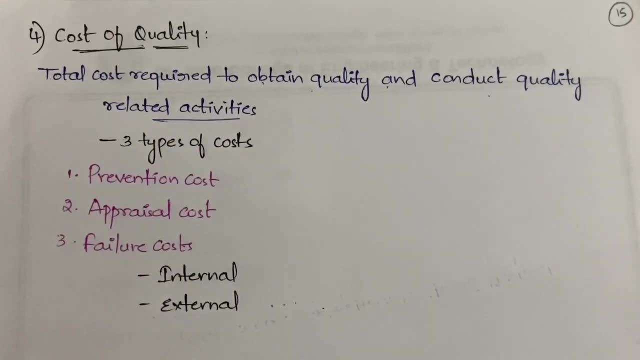 of quality. so, in cost of quality, it is nothing but the total cost which is required to obtain the quality and conduct quality related activities. so, in order to obtain, in order to achieve the quality, the cost of quality, the price of quality, in order to perform quality related tests, that is, in order to perform the quality related activities or tasks. 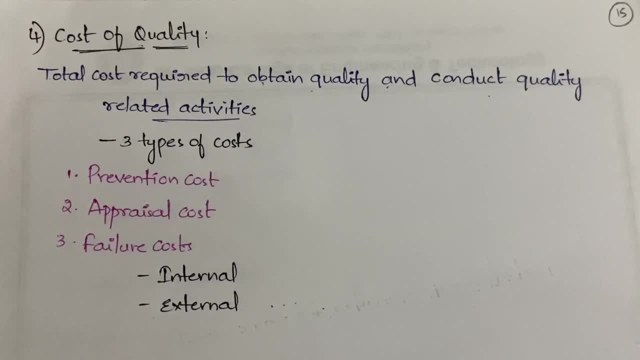 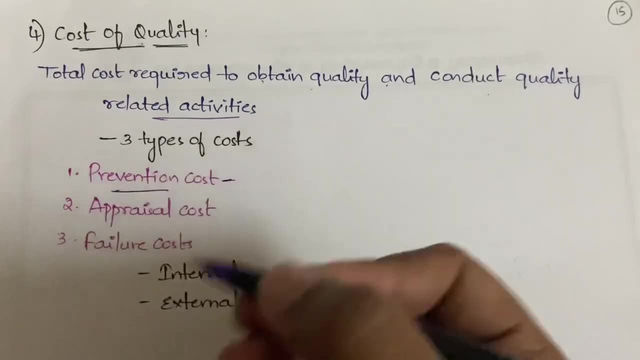 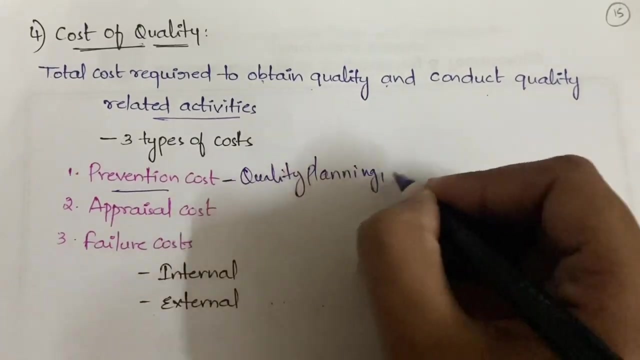 how much money you are spending, how much cost is required. that is, what cost of quality means. okay, in this we have some things like we have the prevention cost. so what will come under prevention, prevention cost? so what will come on a prevention cost is a quality planning, quality planning and formal technical reviews, and 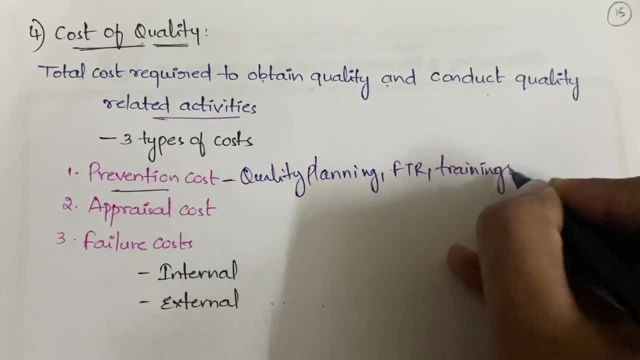 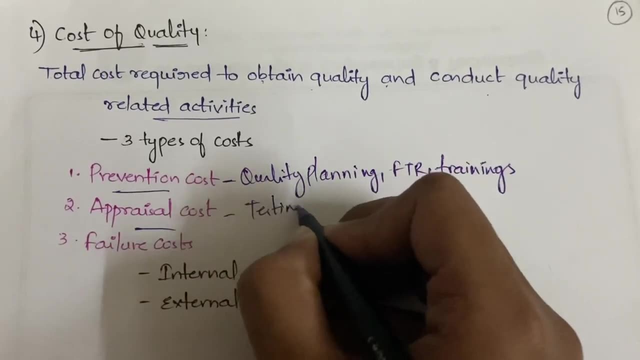 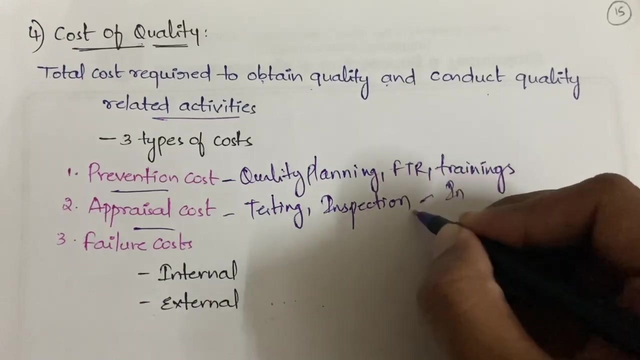 and the trainings, all these will come under the prevention costs. okay, so next comes the appraisal cost. in appraisal cost you will have testing and you will have in process and inter-process inspection. you will have inspection and that inspection types. it could be in process inspection or it could be inter-process inspection. in process inspection is nothing but within the process.